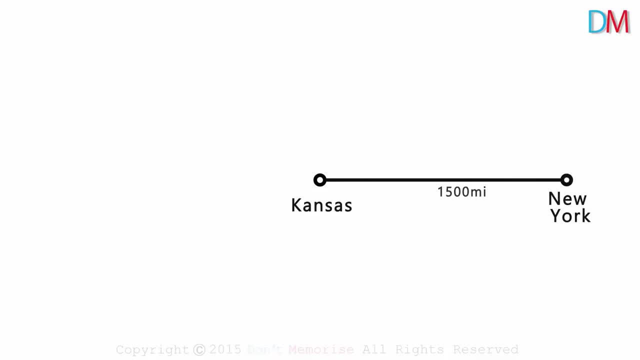 You have New York, 1500 miles to the east, and California, 1500 miles to the west. One day you decide to meet your friend in New York. You leave in the morning and after having covered around 400 miles, you get a phone call. 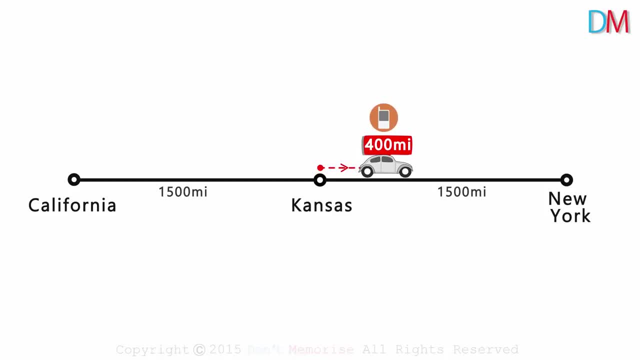 You stop your car and answer the call. Wah, You've been called to Mountain View, California, for an important meeting. You decide to rush towards California. It all goes well. You finish your meeting in California And then you're on your way back home. 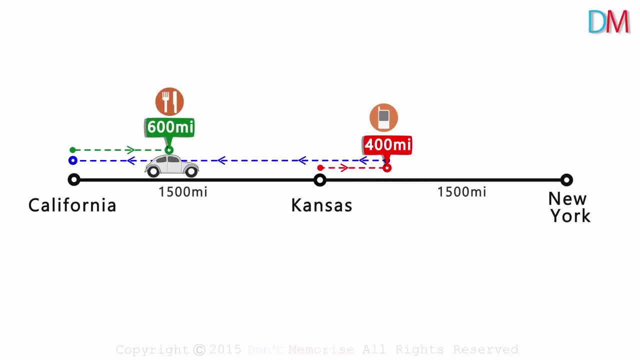 After covering around 600 miles, you decide to stop for lunch, And then you start wondering about two things: First, how far away from home are you placed, Which means how far are you from Kansas, And second, what's the total distance you've covered? 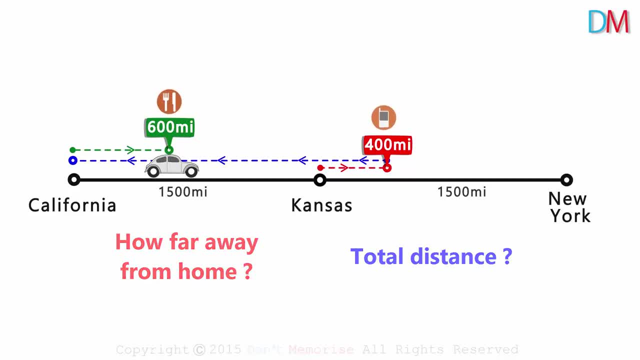 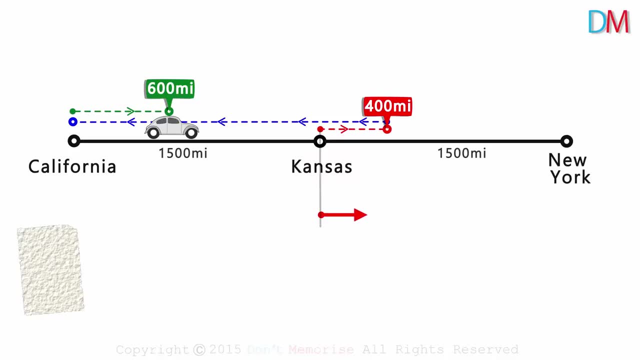 Yes, how much distance have you covered in travelling back and forth? Let's note down the sequence of events, assuming your home as the reference point. First You travelled 400 miles to the east- This distance is 400 miles- And then, from this point, you travelled to California. 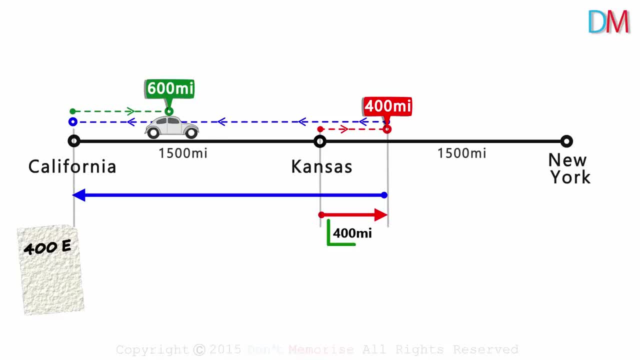 What would be the distance from this point to California? It would be this distance plus this distance, That would be 400 plus 1500, 1900 miles towards west, And from California you travelled 600 miles to the east. This distance is 400 miles. 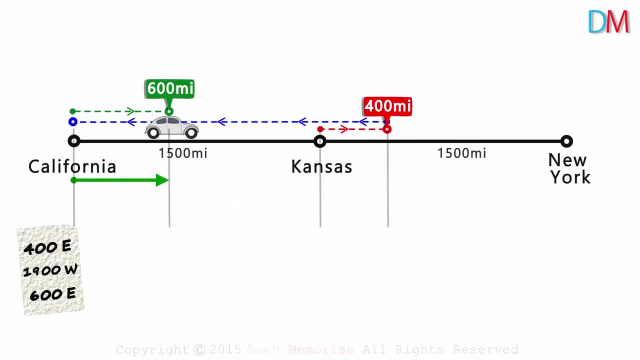 This entire distance is 1900 miles And this distance is 600 miles. Let's talk about the first question that came to your mind: Where are you in relative to Kansas? To understand that answer, think of this as a number line. 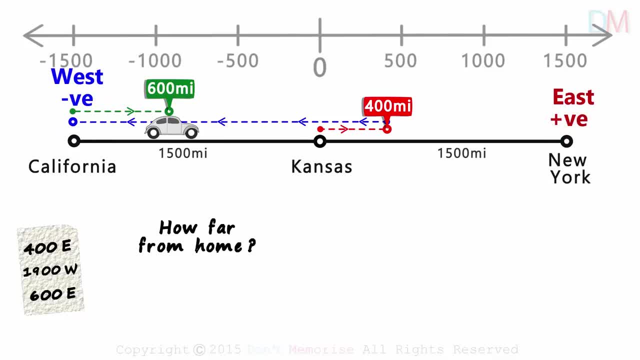 A number line in which east is positive and west is negative, 400 miles to the east will be positive 400.. Then 1900 miles to the west would be negative 1900. And 600 miles to the east would be positive 150. 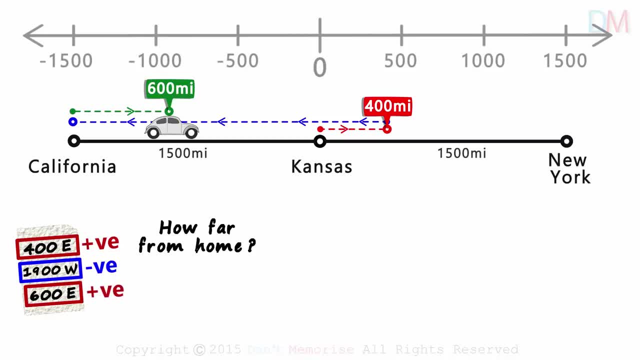 So where are you? You've travelled over 400 miles. This distance is 600 miles positive 600. What would these numbers add up to? East is positive, so we write 400.. As West is negative, we subtract 1,900 and then add 600 again, as it's in the positive direction.